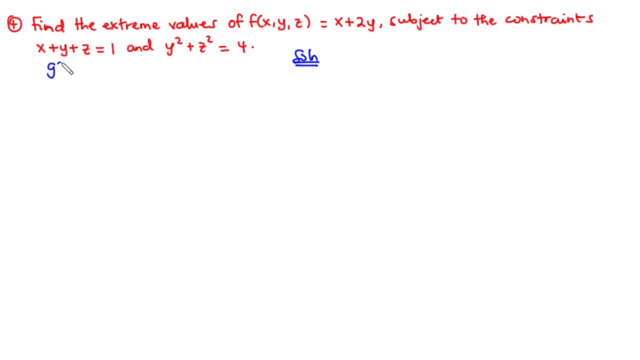 So we are going to let the first one be g of x y z and then the second function be h of x y z. So we are going to find fx, fy and then fz, and then we do the same for g and then h. 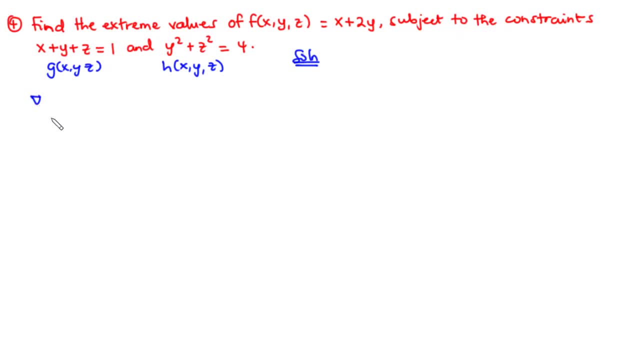 Notice that at the end we are going to obtain the vector equation which is given by: the gradient of f is equal to lambda times the gradient of y, So g plus mu times the gradient of h. So for fx we are going to have 1,, fy we have 2, and then fz we are going to have 0. 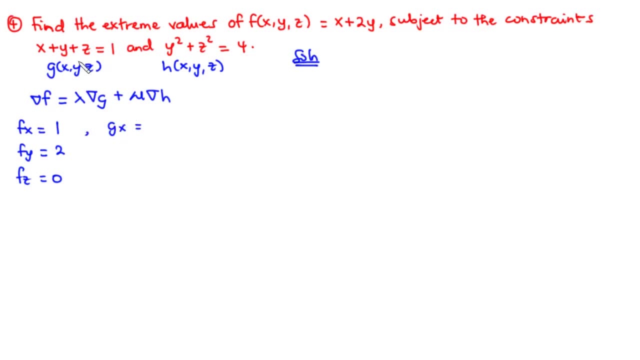 Now also for gx, gx, we are going to have 1, we have gy also to be 1.. And then gx- gx also to be equal to 1.. And then, lastly, for h, we have hx to be 0,, we have hy to be 2y, and then hz to be 2z. 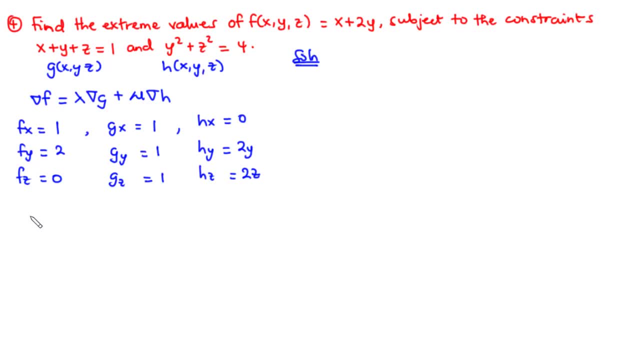 Now the next thing we are going to do is to compare corresponding components and make equations out of them. So we are going to have fx, So we have gx, We have 1. And that is equal to lambda times gx, And that is lambda. 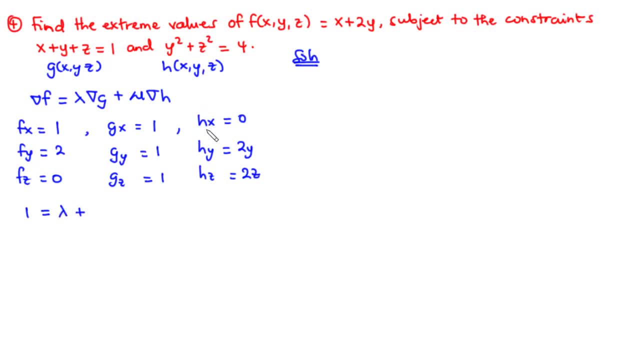 And then plus mu times hx. Now hx is 0,, so it goes to 0.. So it means that we have 1 equals lambda, and that is equation 1.. And then we move on to the next one. We have 2 equals lambda times 1,, which is still lambda, plus 2y times mu. 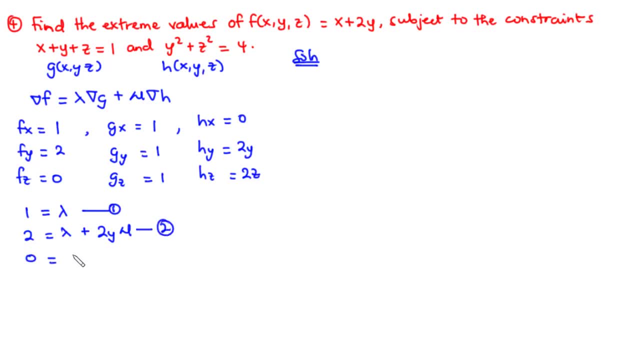 We call that equation 2.. Next we have 0, equals lambda, times 1,, which is still lambda, and then plus 2z mu. That is equation 3.. And then we have the two constraints. We are going to have x plus y plus z, equals 1.. 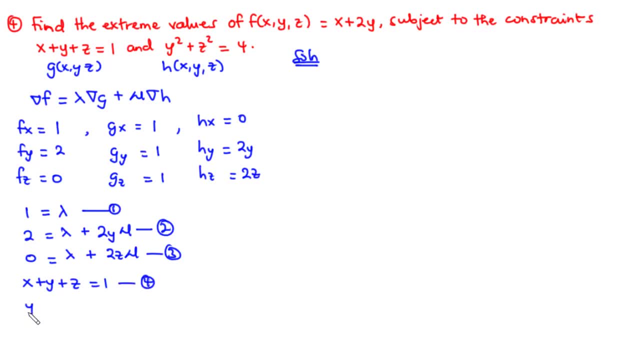 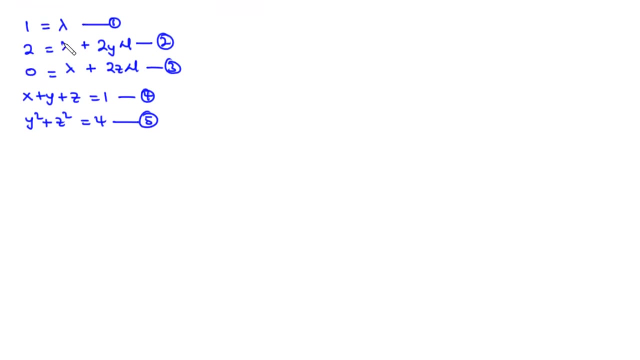 That is equation 4.. And then we also have y squared plus z squared equals 4.. And that is also equation 5.. Now, the first thing we need to do here is we need to realize that we have lambda equals 1.. 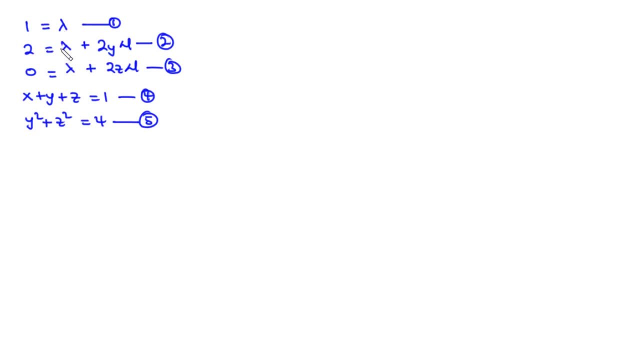 Now, in that case, we can decide to put lambda equals 1 into equation 2 or equation 3.. However, equation 3 looks a bit simpler, So you are going to put lambda equals 1 into equation 3.. So by so doing, 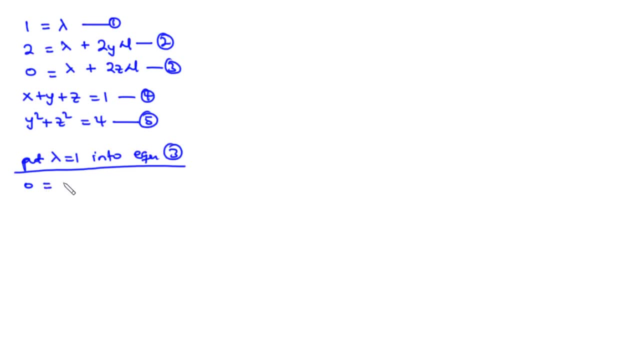 we are going to have 0 equals 1.. Now we can simply make this negative: 1. We transpose lambda to the left-hand side, So that will be equal to 2 times z times mu. Now we are going to obtain an expression for mu. 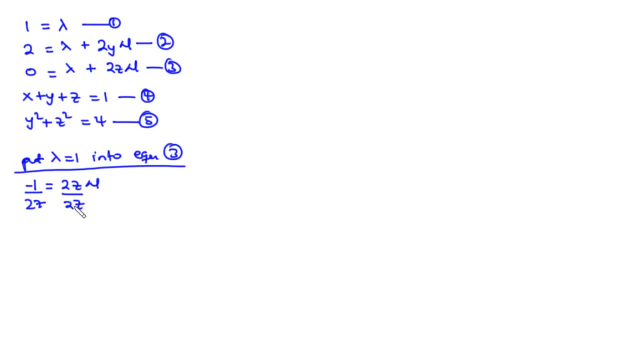 So we divide through by 2z and then we have mu to be equal to negative 1 over 2z. So this is an expression for mu. Next, we are going to put mu into equation. We are going to substitute mu into equation 2.. 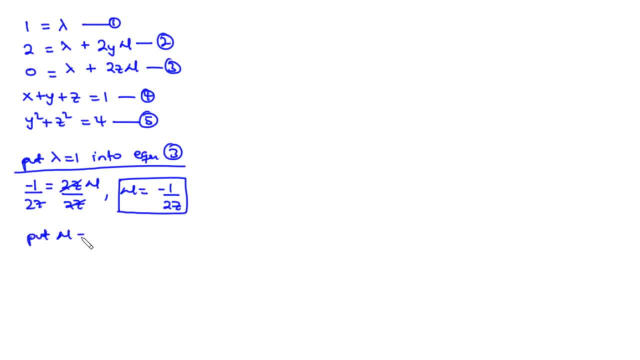 So we put mu equals negative 1 over 2z into equation 2.. By so doing we eliminate mu and then we can then consider equation 4 and 5.. So from equation 2, we are going to have 2 equals lambda is 1.. 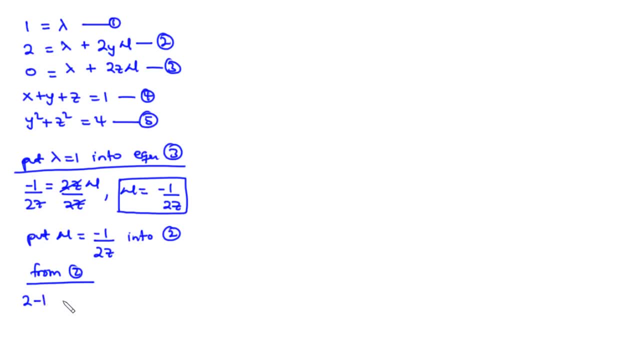 So we transpose 1 to the left-hand side, So we have 2 minus 1, and that's equal to 2 times y times mu. And then mu is given as negative, 1 over 2z. So we have 1 on the left-hand side and that is equal to. 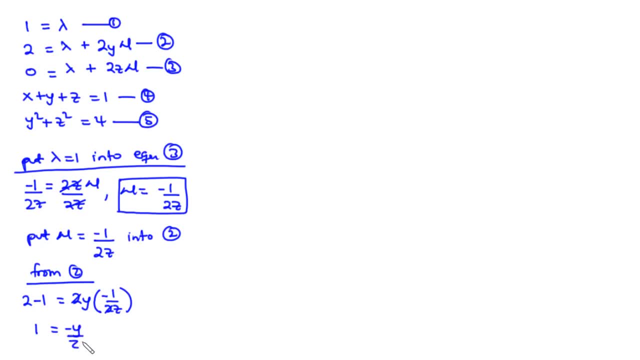 2 cancels out 2.. We are left with negative y over z. Therefore, we have z to be equal to negative y. So this is an expression for mu. So this is an expression for mu. This is the value of. 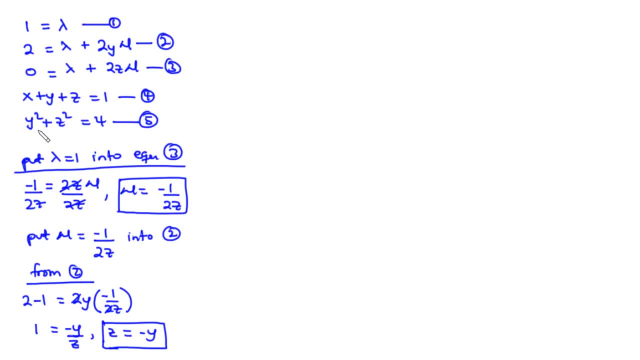 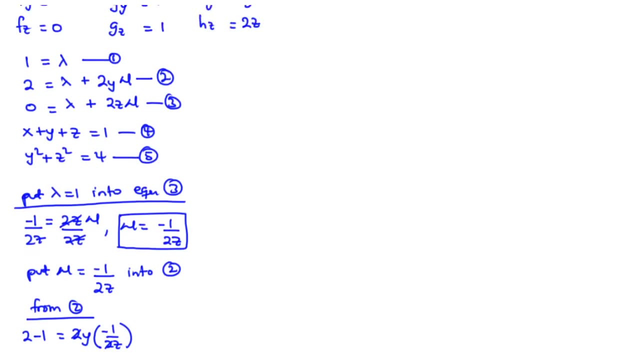 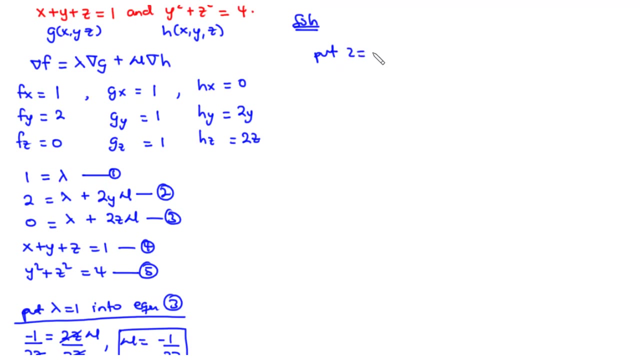 Or this is an expression for z. Now, since we have y squared plus z squared equals 4, then we can put z in here, We can put z in there. So we say that we are going to put z equals negative y into. 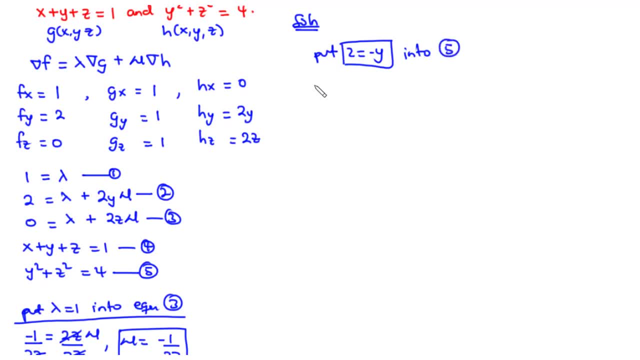 equation 5.. Into equation 5. So that we have y square plus negative. y square equals four. so this becomes two y square equals four. we divide through by two and then we have y square equals two. so we take the square root of both. 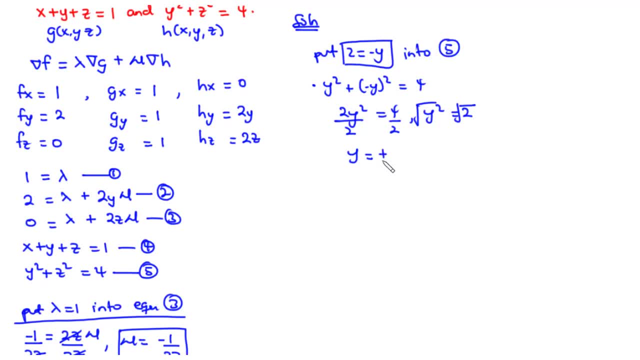 sides. and then we have y equals plus or minus root two. so this is the value of y now, for y equals plus or minus root two. then we can have z also to be equal to negative into bracket plus or minus root two, and that is still plus or minus root two. so this is. 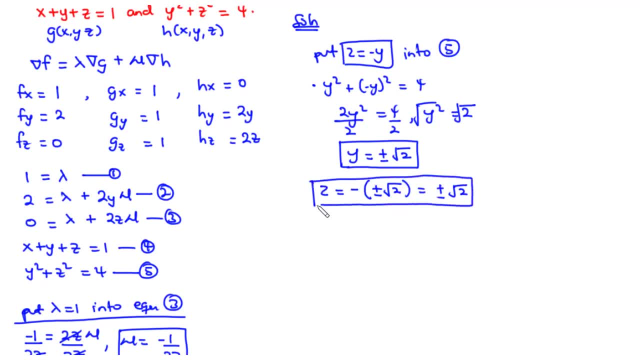 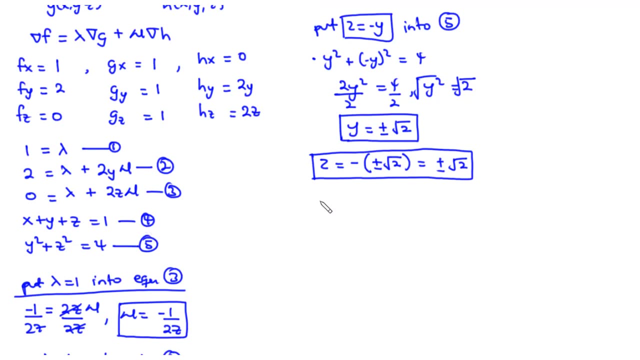 also values of z. now we have values of y, we have values of z. we need to find the values of x. so to find the values of x, we can use equation four. so from equation four we have x plus y plus z equals one. now, because we have different values of 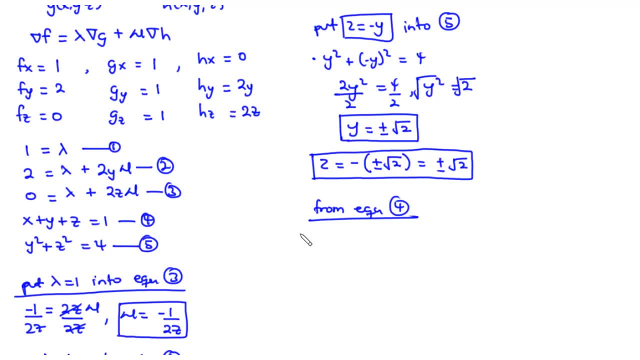 y and then z. we need to consider that, for y equals root 2, we have z to be equal to. z is equal to negative y, so we can have this to be negative root 2, and thus if we want to find the value of x, then x will simply be equal to. we have 1, and then minus y, minus z, so we have x to be. 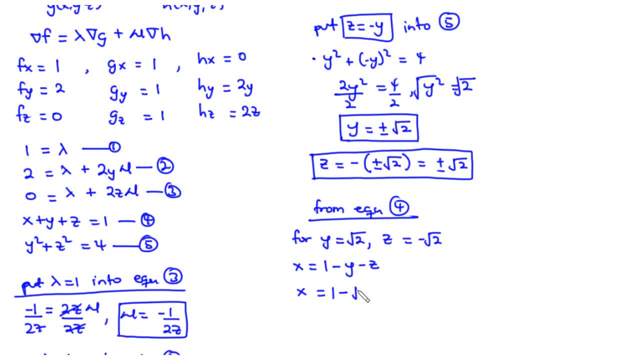 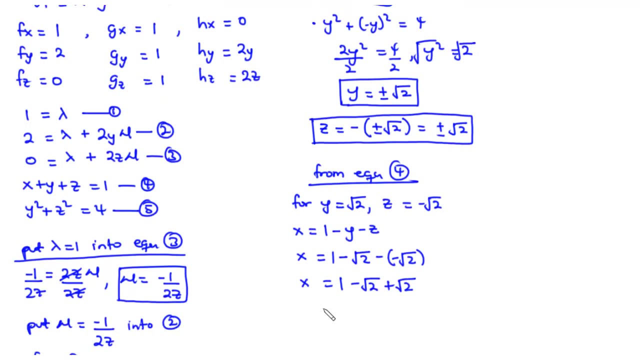 equal to 1 minus y, so minus root 2, and then minus negative root 2. so this becomes: x equals 1 minus root 2 plus root 2, and thus we have x to be equal to 1, so x is equal to 1, and then 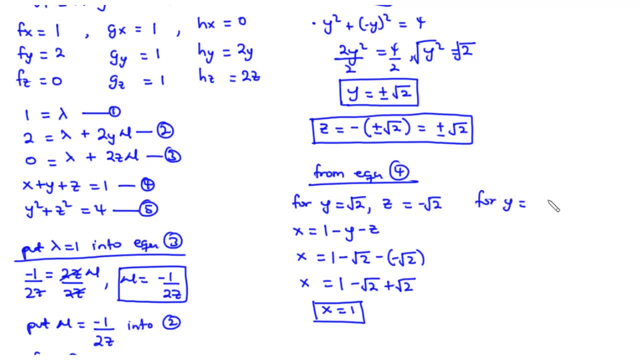 for y equals negative root 2, z will be equal to positive root 2. therefore we have x to be equal to 1 minus y minus z, and that is equal to 1 minus negative root 2. so minus negative root 2 and then minus. 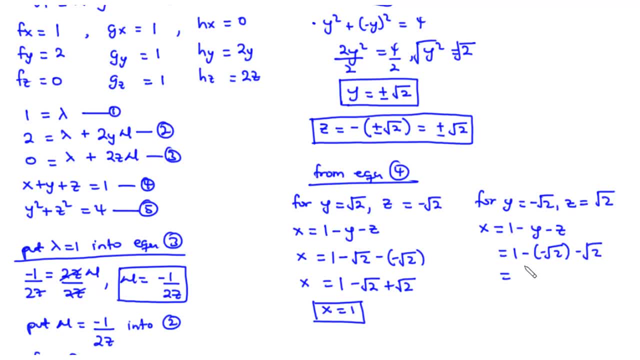 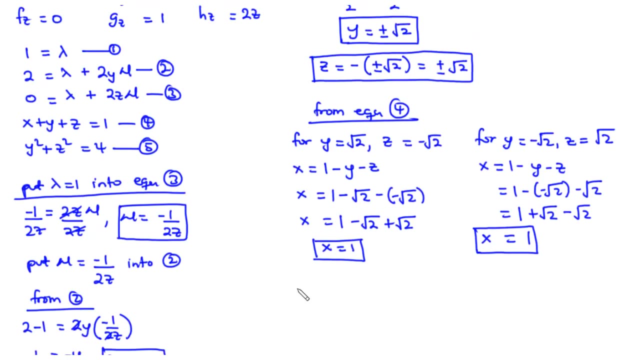 negative root 2, so it becomes 1 plus root 2 minus root 2, and thus we have x also to be equal to 1.. so therefore, we have two points, which are 1 root 2- negative root 2 and 1 negative root, 2 root 2. so you need to find the value of the function at this point. 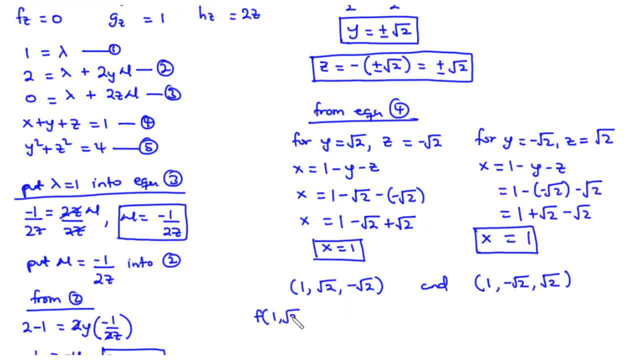 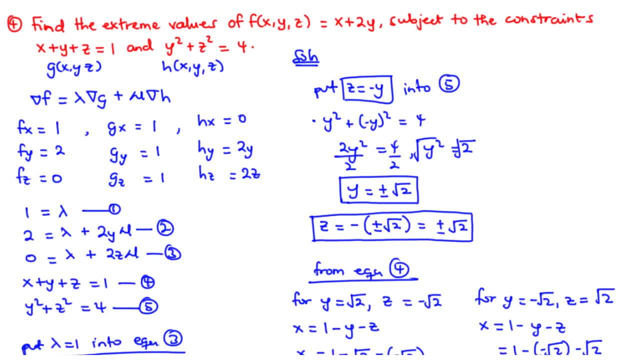 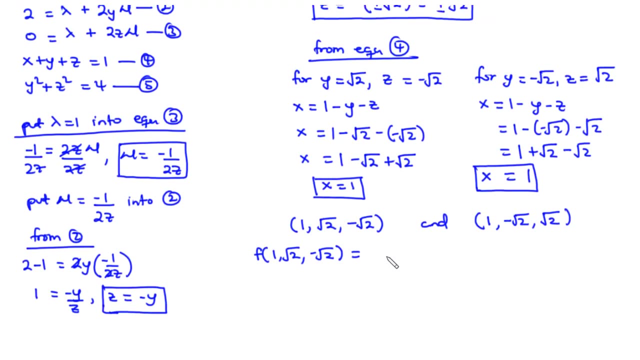 so f of 1 root 2, negative root 2. we have the function giving us x plus 2y, x plus 2y, so x plus 2y. let me write it somewhere here: f of x y, z is equal to x plus 2y. therefore we have x to be 1 plus 2 times root 2, so this is equal to. 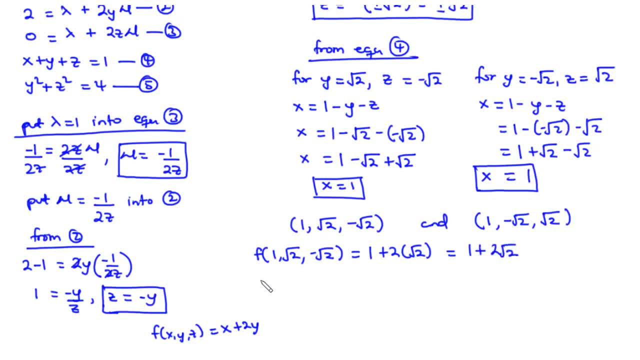 1 plus 2 root 2 and then for f of 1 negative root 2 root 2, we are going to have 1 plus 2 times 2x times negative root two. so that will be one minus two root two. so therefore we are going. 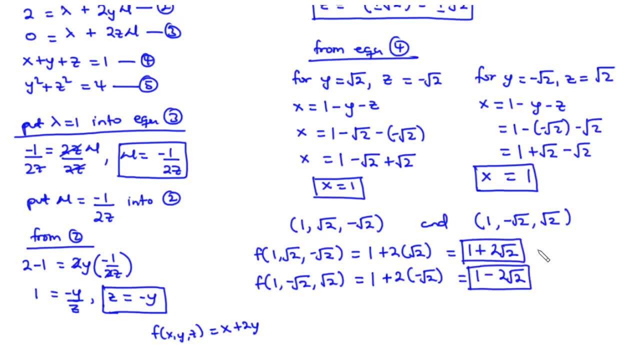 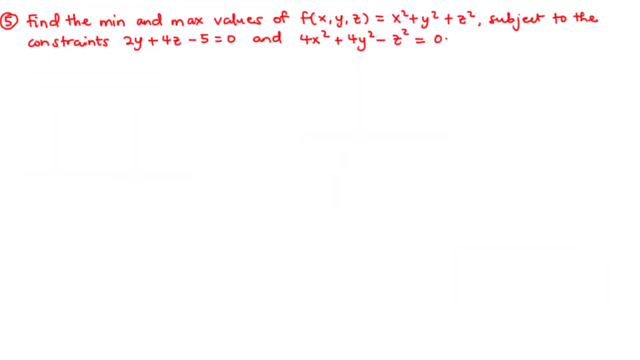 to have one plus two root two to be the maximum value, and then it occurs at the point one root two negative root two, and then one minus two root two becomes the minimum value and also occurs at one negative root two root two. now let's move on to example five in this. 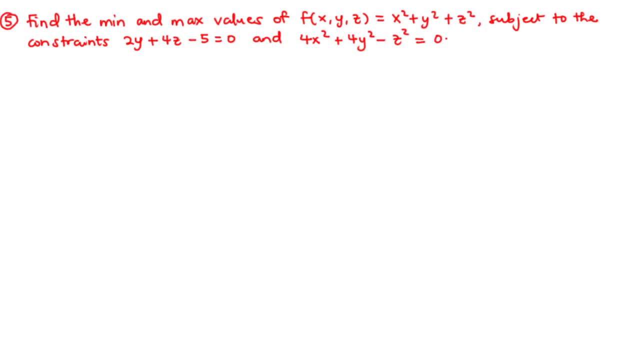 example, we are going to find the minimum and the maximum values of the function f subject to the constraint two y plus four z minus five equals zero, and four x square plus four y square minus z square equals zero. so we obtain the vector equation which is given. 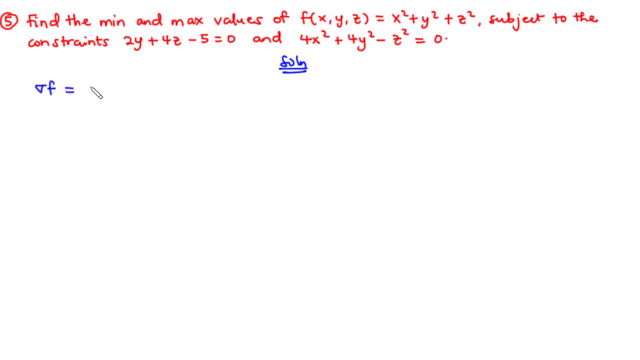 by the gradient of the function f equals lambda times gradient of the function j plus mu times gradient of the function h. so let's find fx, fy and then fz, and then we do same for j and then h. so we have fx that's equal to two x, fy is also two y, and then fz is also equal. 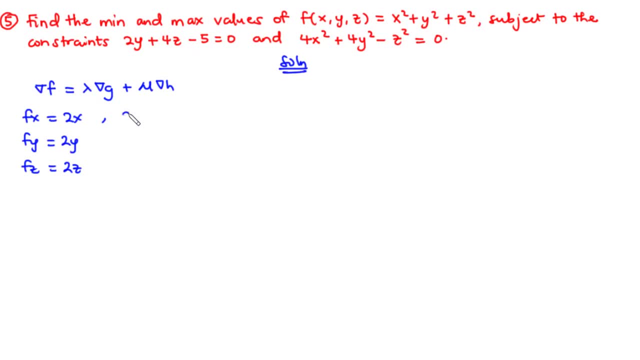 to two z. now we also for j, we have j x. now here we don't have any x components, so j- x equals zero. we have j y to be two and then j z to be equal to four, and then for h, h, x equals. we have: 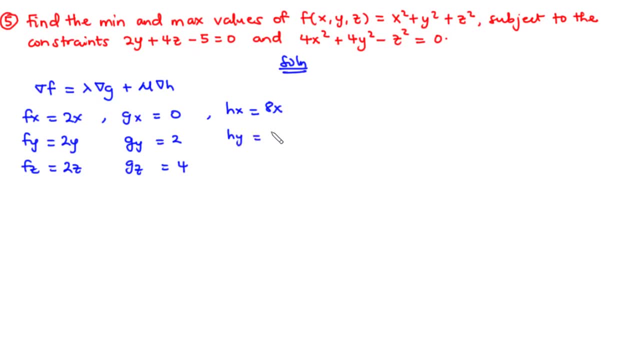 8 x. h y equals 8 y, and then h z equals negative. So at this point we are going to form equations taking into account corresponding components. So we have fx, which is 2x, equals lambda times jx, So that is 0 plus mu times hx. 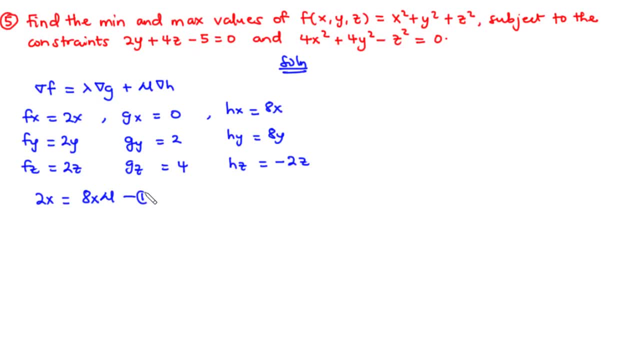 So we have 8x mu, That is equation 1.. Next we have 2y- equals 2 lambda plus 8y mu. That is equation 2.. And then we also have 2z- equals 4 lambda minus 2z mu. 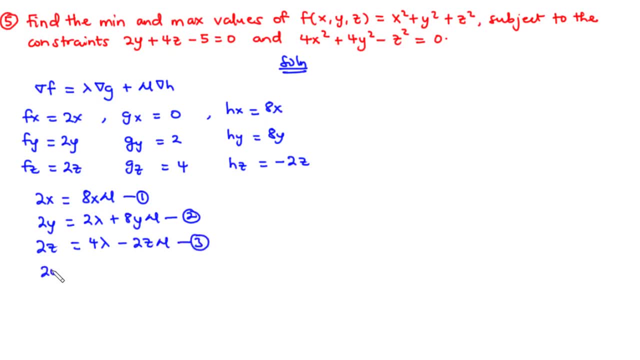 That is equation 3.. And then we have the constraints: 2y plus 4z equals 5. We transpose negative 2. And then we put 5 to the right hand side, So that is equation 4.. And then, for the fifth equation, we have 4x squared plus 4y squared minus z squared equals. 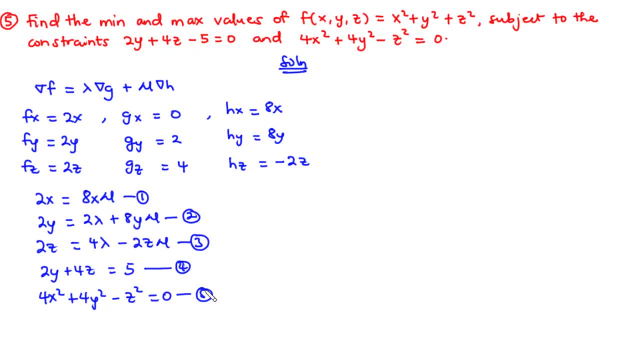 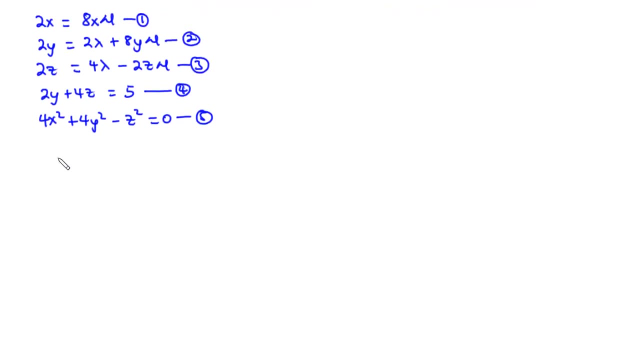 0. Now what we are going to do here is we are going to consider equation 1, because it looks simpler, and then we transpose 8x mu to the left hand side, So we are going to have to have that is from equation 1. we have 2x minus 8x times mu equals 0, the greatest common factor. 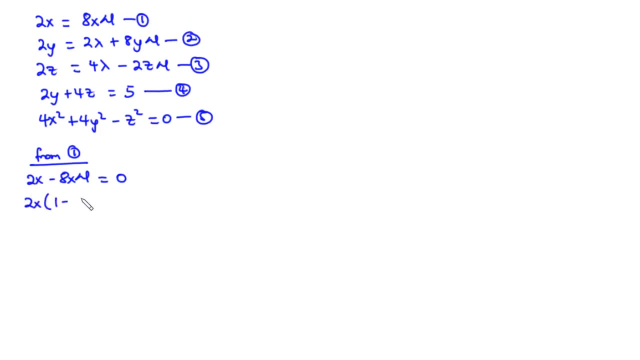 is 2x. so 2x on the outside, 1 minus 4 times mu inside, equals 0. we have 2x equals 0 and thus x is equal to 0. so we have x equals 0. we don't really care about the value of mu. 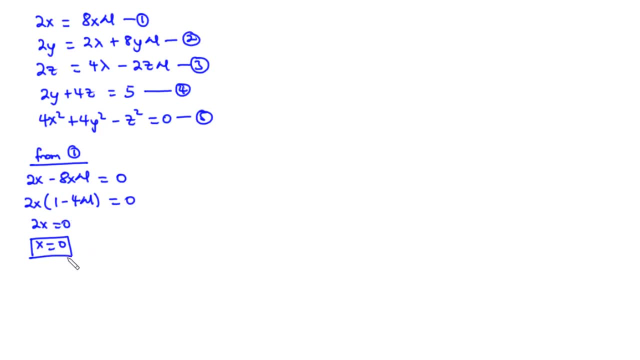 now we are going to put x equals 0 into equation 5. so we put x equals 0 into equation 5 and then we are going to have 4 times 0 square plus 4. y square minus z square equals zero. so this becomes four y square minus z square equals zero. now, at this point we can represent: 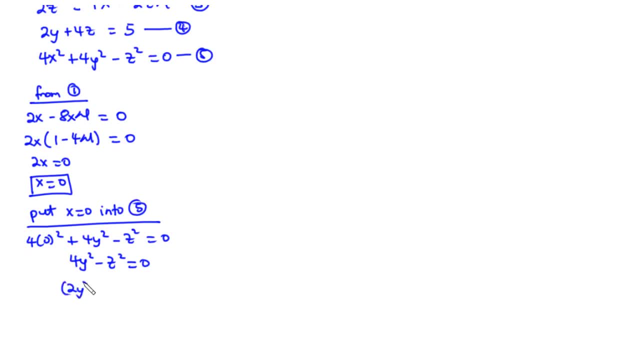 the expression on the left hand side as two y all square minus z square. therefore, we have difference of two squares on the left hand side, so that we can represent this as 2y minus z, and then times 2y plus z equals 0.. so we are going to have z equals 2y or z equals negative 2y. 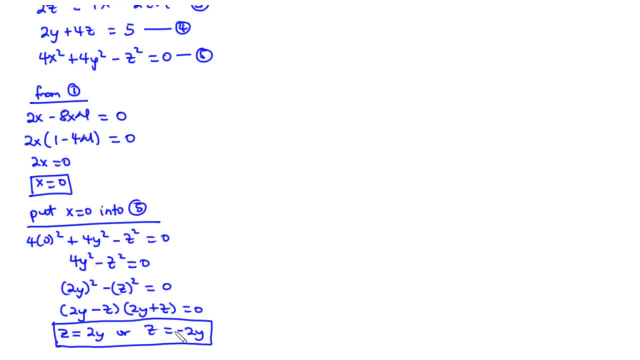 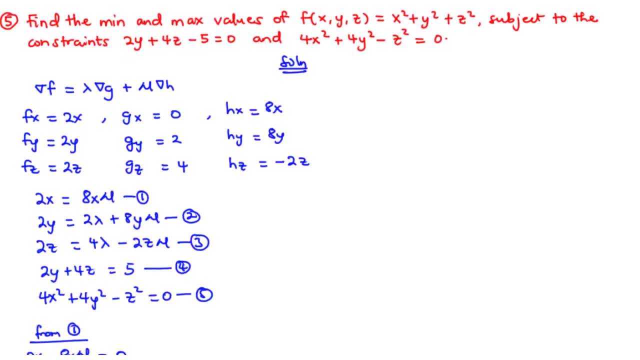 so the next thing is: we are going to substitute z equals 2y, z equals negative 2y into equation four, into equation four. so from equation four, from equation four, we have two y plus four z equals five. so we have z equals negative two y, z equals two y. so for z equals negative two y, 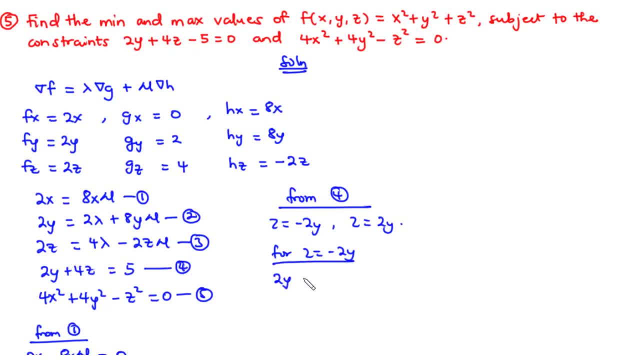 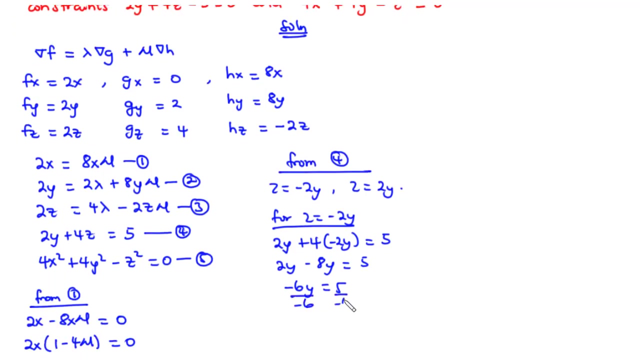 from equation four, we are going to have two y plus four times negative two y equals five. so this becomes two y minus eight, y equals five. and then we have negative six. y equals five. we divide three by negative six, negative six, we have y to be equal to negative five over six. 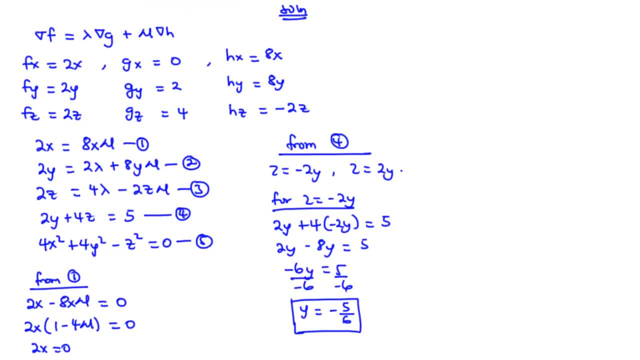 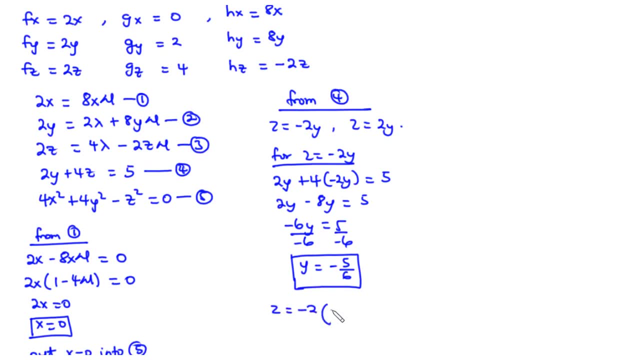 now, if y is equal to negative five over six, then what this primarily means is that z is equal to negative. two times negative, five over six. two goes here once. two goes here. three times negative, negative, positive. therefore, we have z to be equal to five over three. this is the value of z, and then for z, 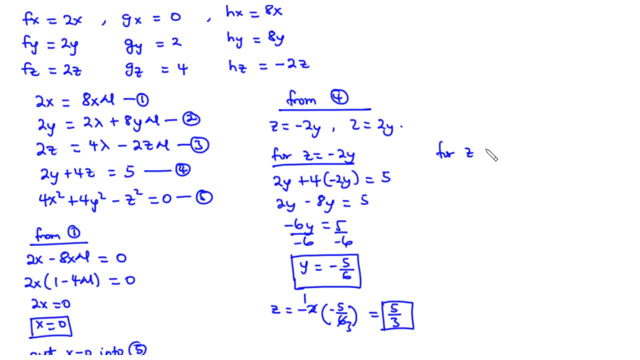 for z also to be equal to two y, then we are going to have from equation four, two y plus four times two, y equals five. so this becomes two y plus eight. y equals five. we have ten y equals five. we divide through by 10 and then we have y to be equal to 1 over 2. y is 1 over 2. therefore we are going to 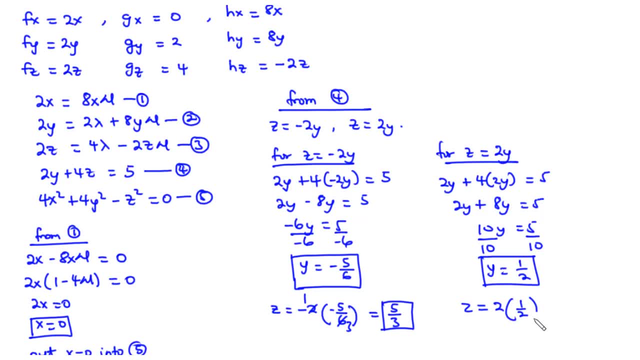 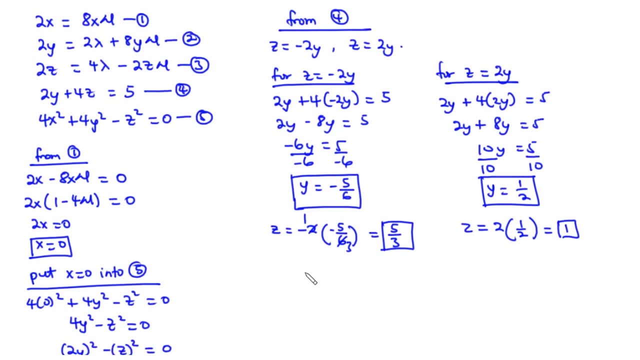 have z to be equal to 2 times y and this becomes 1, so we have the value of z to be 1. therefore, we have two points. the first one is we have x to be 0, 0 for all, and then y to be negative. 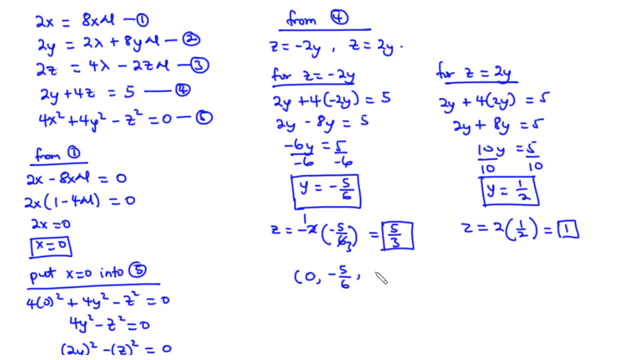 5 over 6 and then z to be 5 over 3 and 0, y is half and then z is 1. now let's try to find the value of the function at this point. so we have f of 0 negative, 5 over 6, 5 over 3, and that's equal. 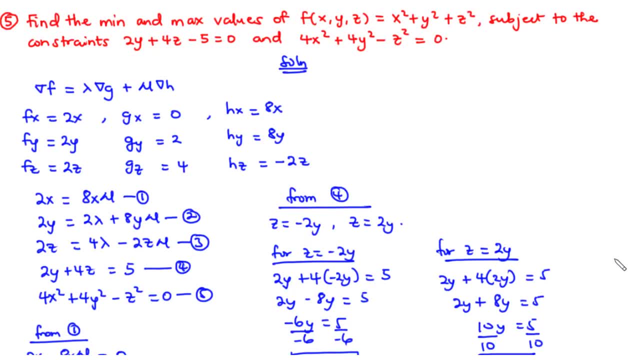 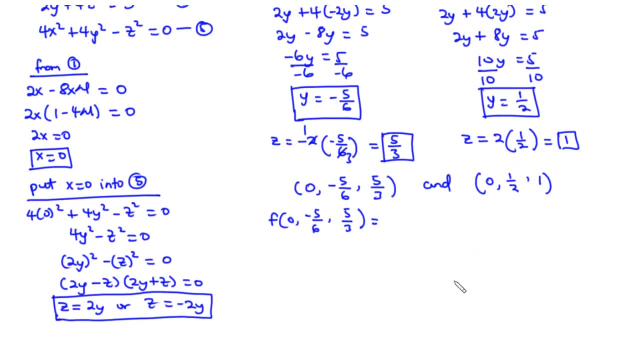 to. we have the value of the function to be x square plus y square plus z square, x square plus y square plus z square, so 0 square plus negative 5 over 6 square plus 5 over 3 square, so this becomes negative 5. so this this is 0 plus negative 5 square is: 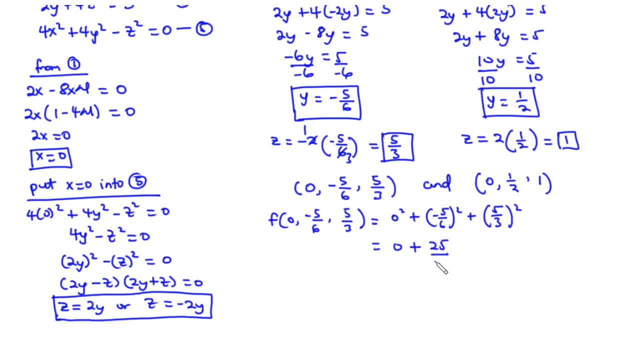 negative 5 and then this becomes negative 5 plus negative 5 over 9. so we have lcm to be 36. 36 divided by 36 is 1. 1 times 25 is 25. plus 36 divided by 9 is 4. 4 times 25 is 100. therefore, 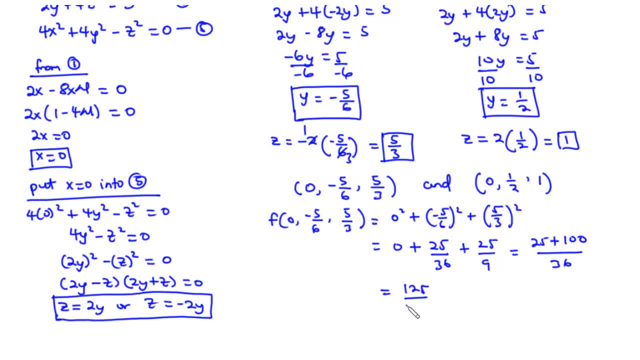 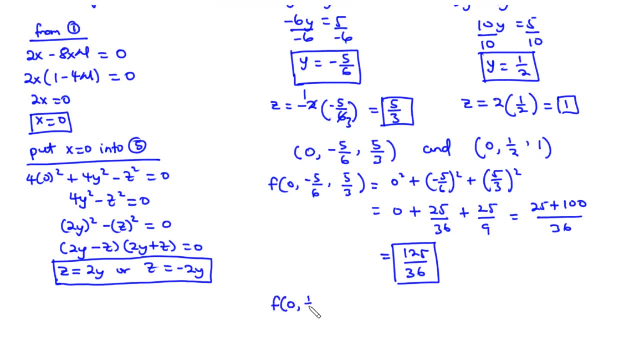 we are going to have 1, 25 divided by 36. so this is the value of the function at the point: 0 negative, 5 over 6, 5 over 3. now for f of 0, 1 over 2, 1. that is also going to be 0 square plus half square plus 1 square, so this will be equal to: 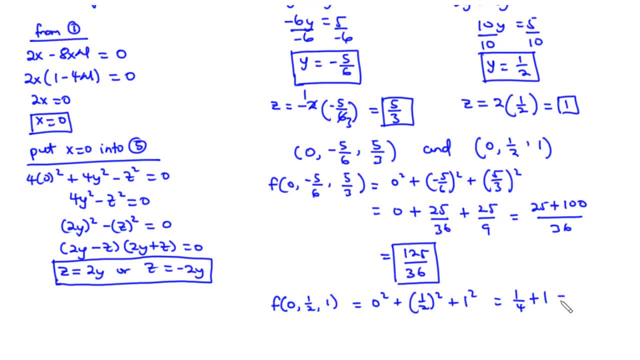 1 over 4 plus 1, and that is equal to. now we can express 1 as 4 over 4, so that's equal to 5 over 4. so this is the value of the function at the point 0: 1 over 2 and then 1, now the highest. 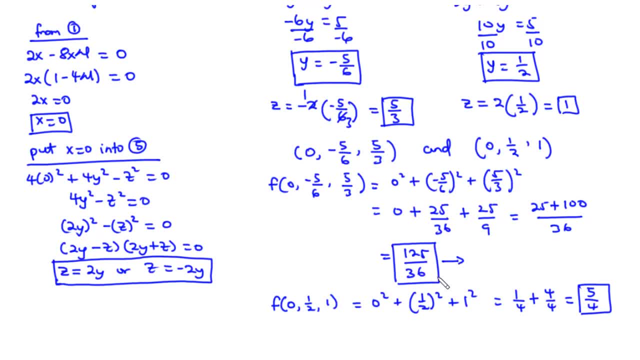 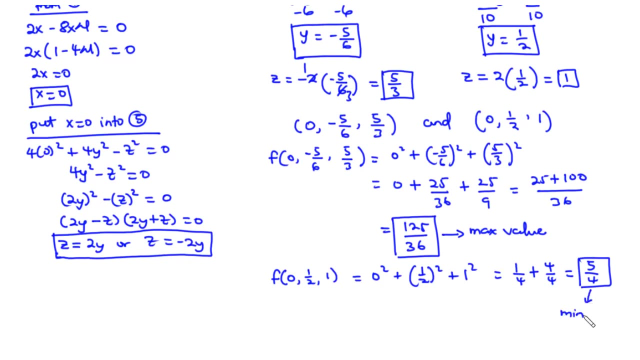 value is 1, 2, 5 over 36, so that is the maximum value and it occurs at the point 0. negative: 5 over 6, 5 over 3, and the minimum value is 5 over 4, and it also occurs at the point 0.